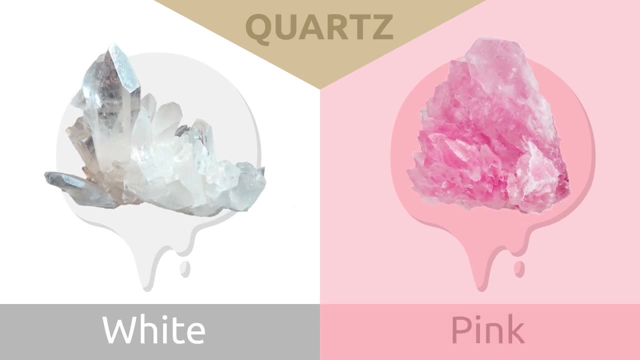 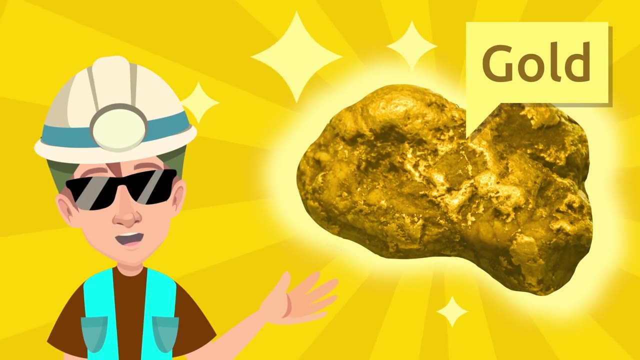 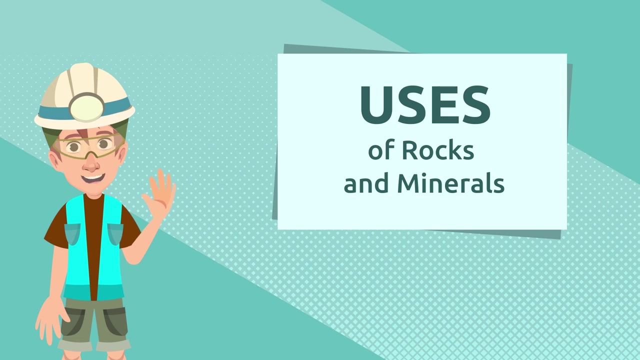 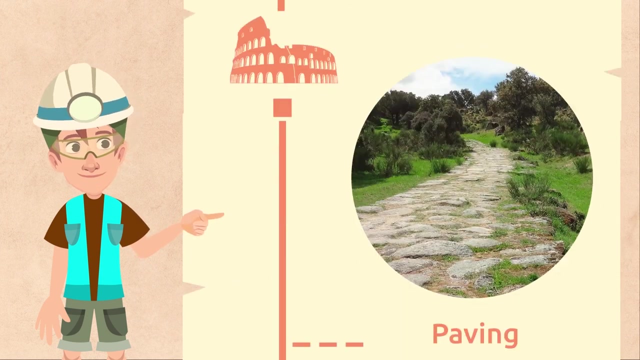 This is a quartz. It can be white or pink, And this is gold, A very shiny material. Since prehistoric times, people have used rocks and minerals for a number of things like making utensils, building their houses, paving or even making beautiful jewelry. 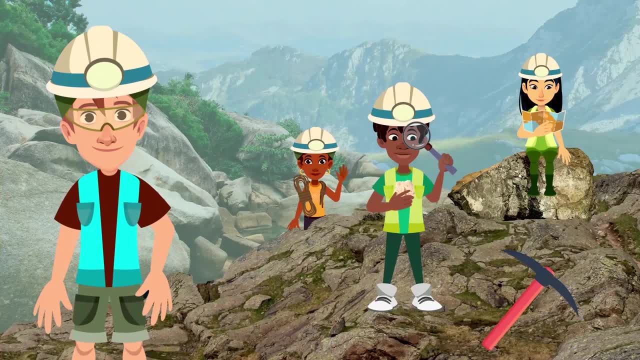 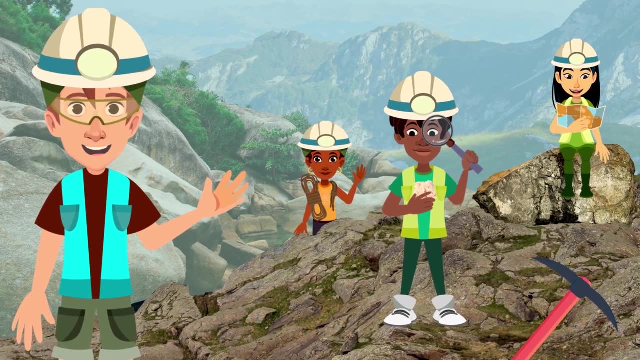 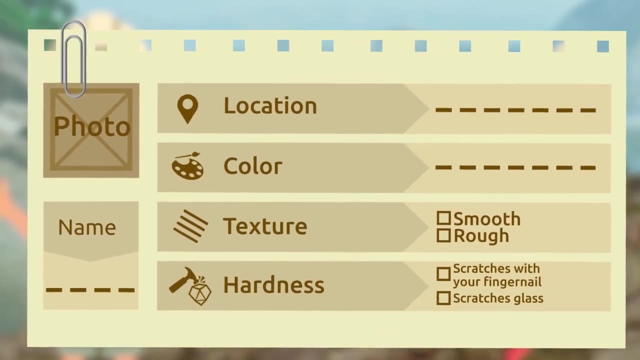 Would you like to try doing this activity? Work with your classmates and put together a rocks and minerals exposition using everything we found on our field trip. You can pick them from different places and study them in class. Tag each rock and each mineral with a label and fill it out yourselves: Name, Photo, Location. 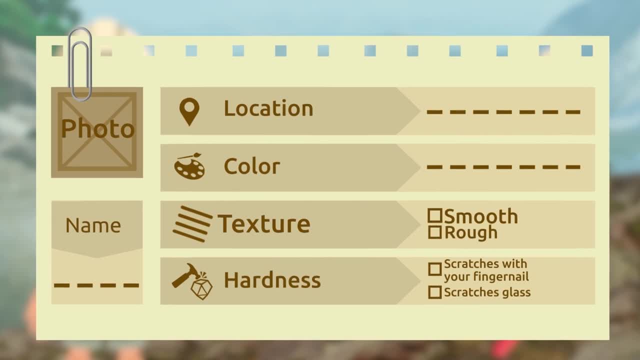 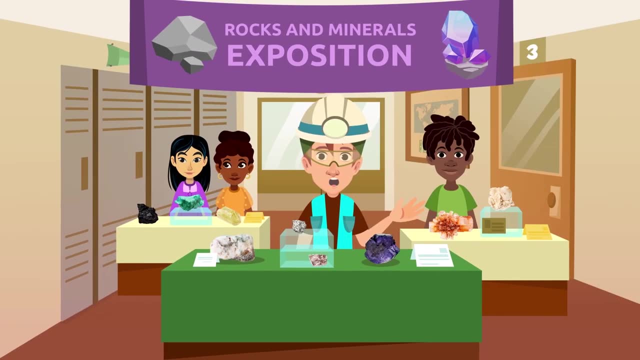 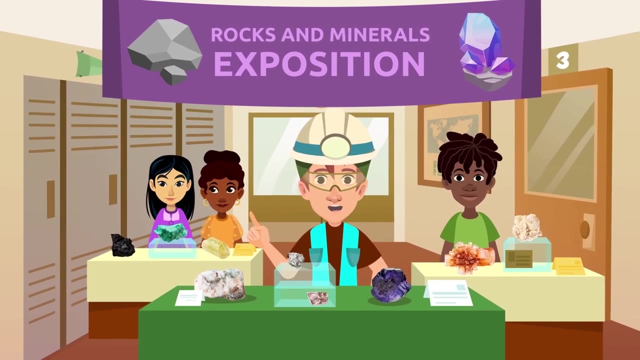 Color Texture: Smooth, Rough, Hardness- Can scratch it with your fingernail. It scratches the glass. The exposition was a huge success. Today we learned that rocks are formed from minerals and that both rocks and minerals are part of nature and the landscape. 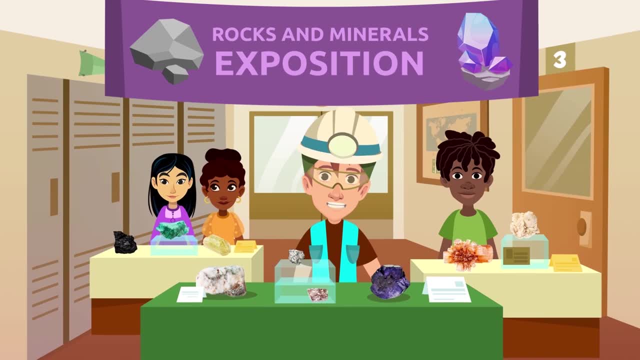 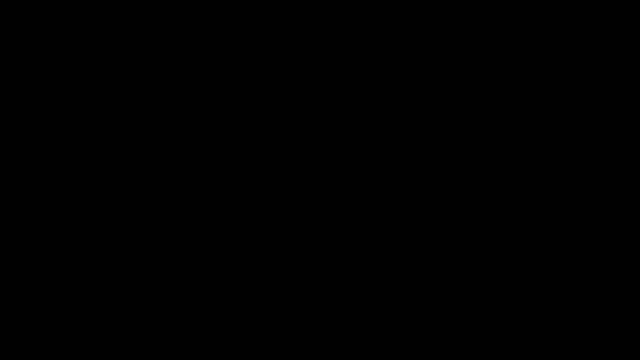 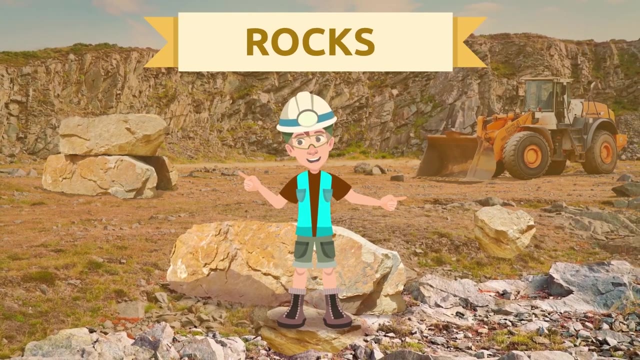 that surrounds us. If you want to learn more about rocks and minerals, watch our upcoming videos. Hello friends, Today we're going on a field trip to learn everything about rocks. I'm sure you'll like it If you're interested in learning more about rocks and minerals. 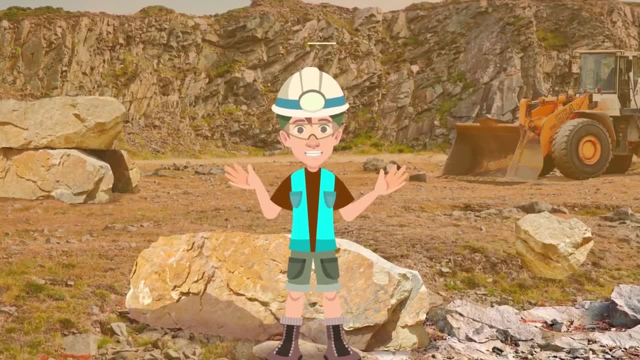 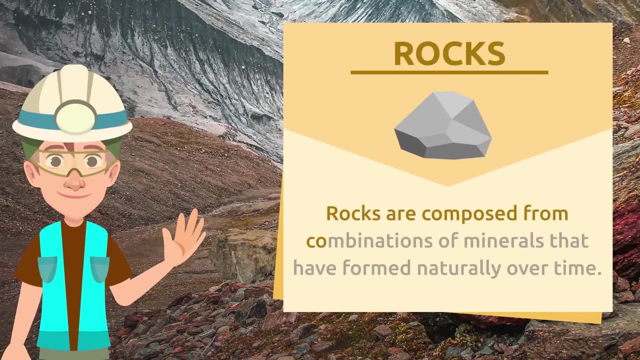 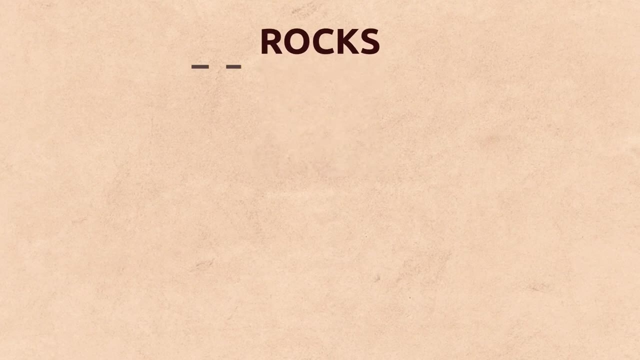 I'm sure you've seen thousands of them, But do you know how rocks are formed and what are their characteristics? Let's find out more about them. Rocks are composed from combinations of minerals that have formed naturally over time. On the basis of their origin, rocks can be classified as igneous, sedimentary and metamorphic. 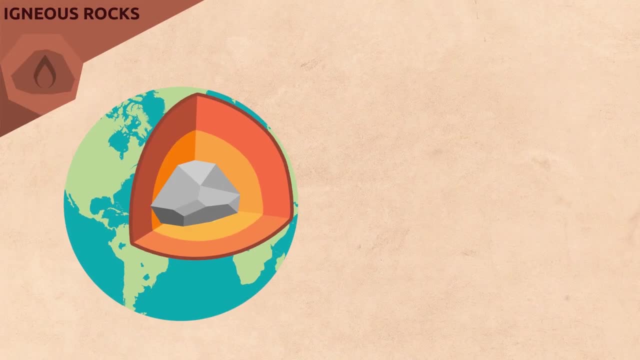 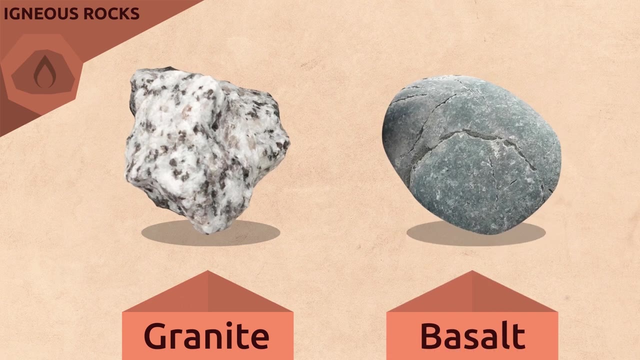 Igneous rocks are very hard rocks. Rocks are formed deep inside the earth. Examples of igneous rocks are granite or basalt. Both are formed from magma which erupts as volcanic lava As soon as it reaches the surface of the earth. 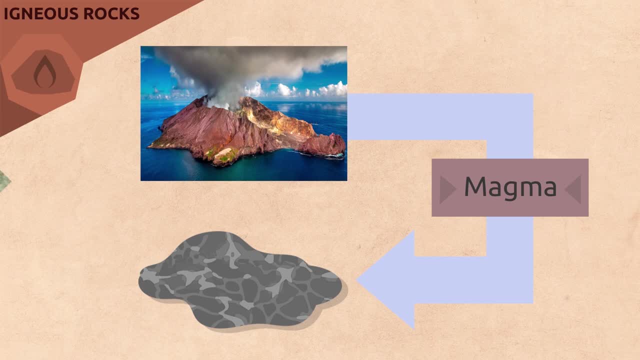 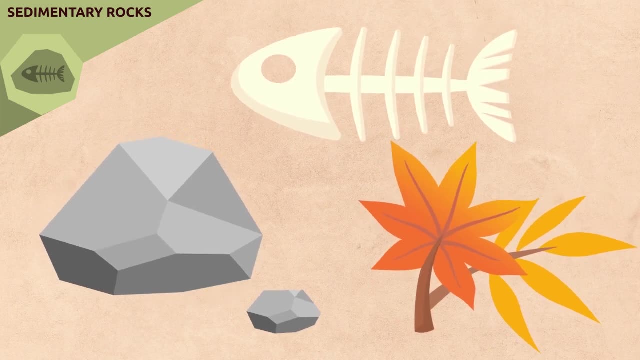 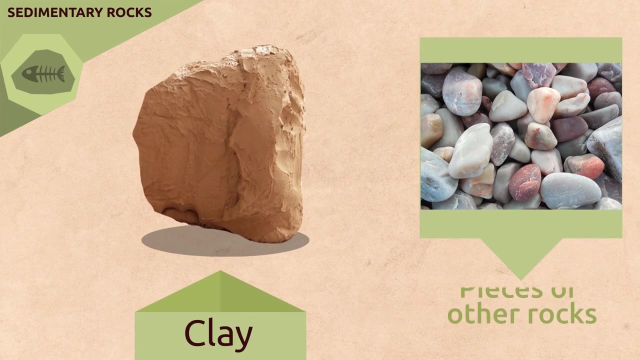 lava cools and solidifies rapidly. Sedimentary rocks are formed from pieces of other rocks or even once-living organisms. Clay, for example, is formed by broken-up pieces of other rocks. Coal and petroleum are formed from the remains of living things like animals. 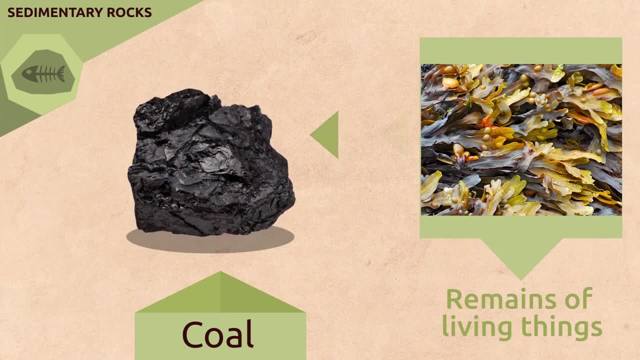 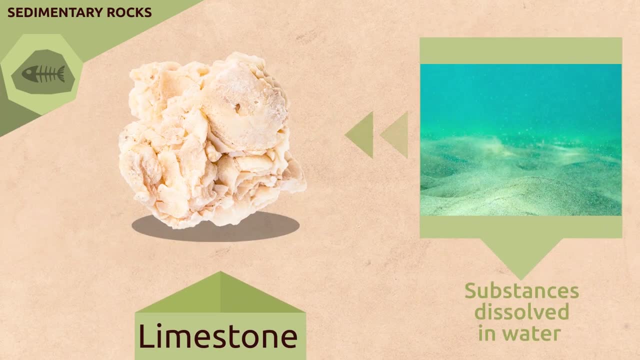 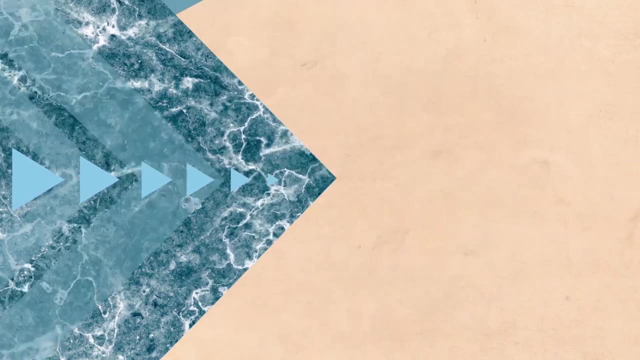 and plants, and from sediment deposits found in marine beds. Limestone is formed from substances dissolved in water And, lastly, metamorphic rocks that are formed by the transformation of other rocks under great pressure or heat are formed from the remains of living things like animals and 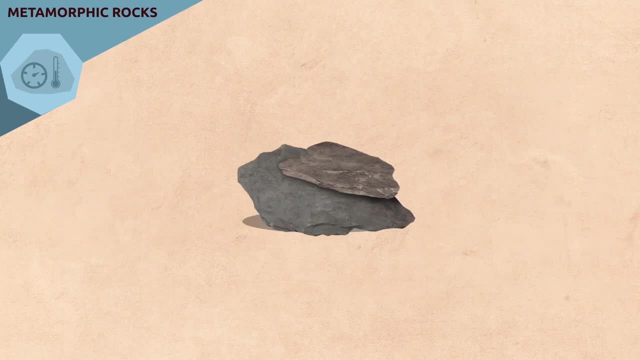 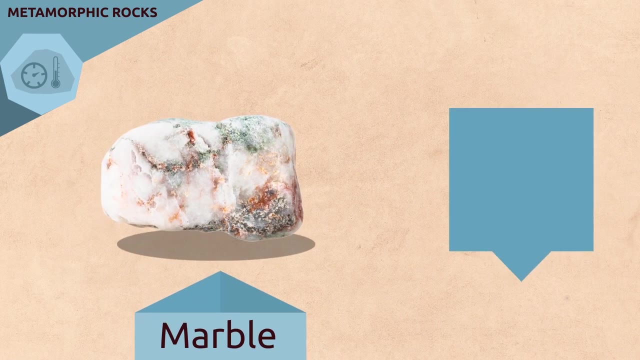 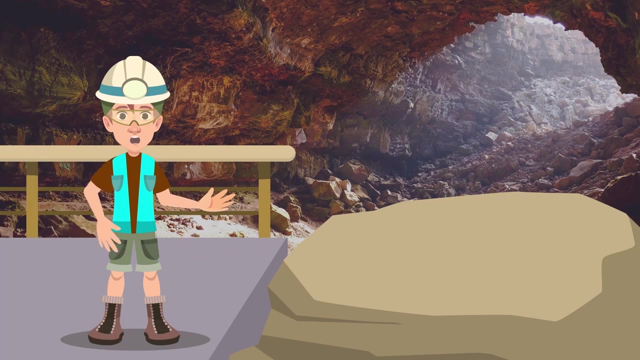 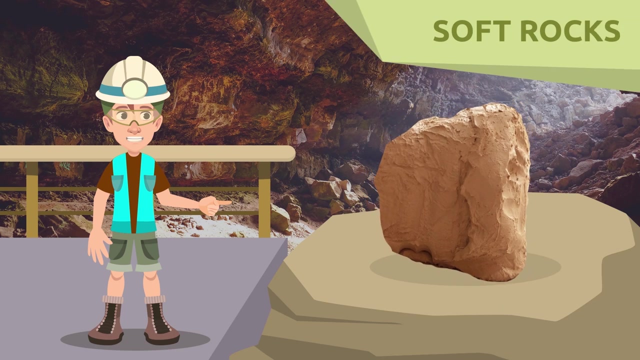 plants Like slate, for example, which is formed from clay, or marble formed from limestone. Rocks can also be classified based on their hardness. That's why we say that there are hard rocks like granite, soft rocks like clay. Petroleum is also considered a rock. 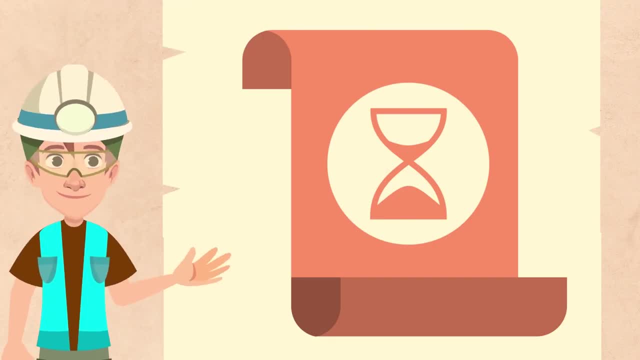 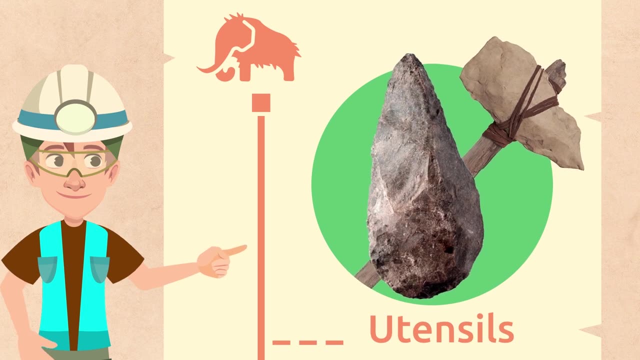 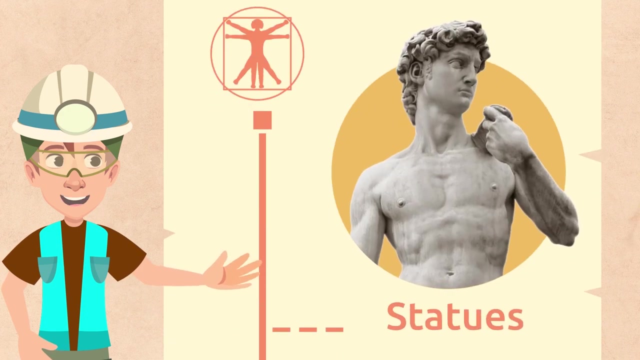 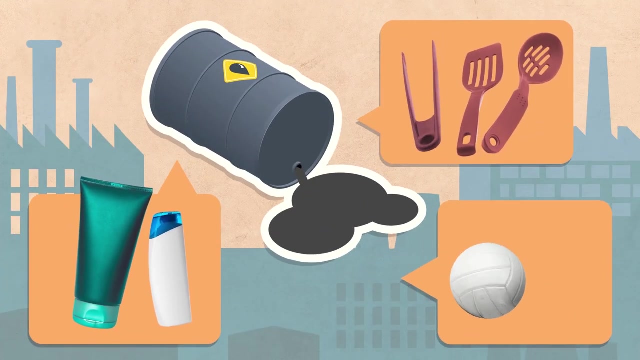 Since prehistoric times, people have used rocks for a number of things, like making utensils, building their houses, paving or even sculpting beautiful statues like this one. Nowadays we use petroleum in different industries for making plastics or coal to generate electricity, And in the past we used it to make wood. But today we use it to make wood. So if you 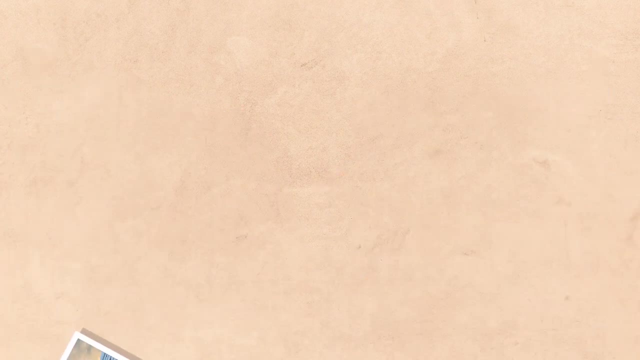 have a few more questions, please leave them in the comments And, of course, those questions can be answered at the end of this video by allergist. We are also looking into the energy consumption and the power of sediment And if you have any questions, 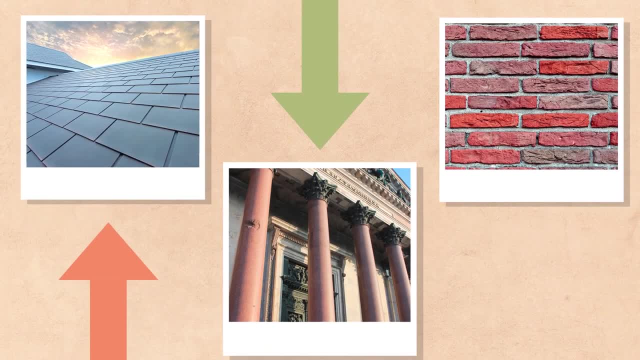 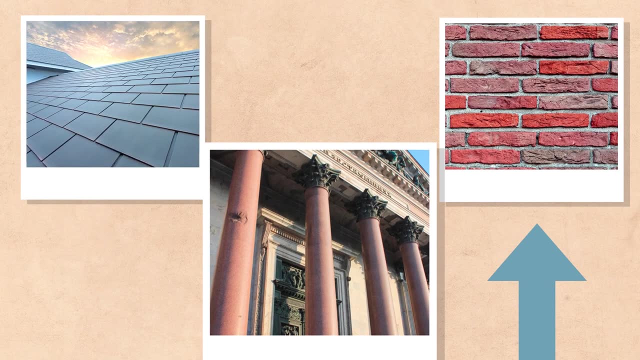 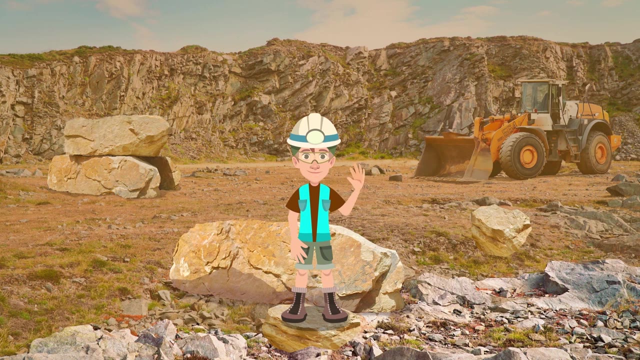 please feel free to post them in the comments. Still to this day, rocks like slate, granite or clay are used in construction. This slate roof, for example, this granite column or a clay brick. What an adventure. Today, we learned that rocks are formed from minerals or even animal. and plant remains. And that, based on their energy content, rocks like clay form minerals. And that only when they are left in the ground or in a environment like this the rocks form minerals. And that, based on their energy content, the rocks are formed from minerals, or even animals and plant. 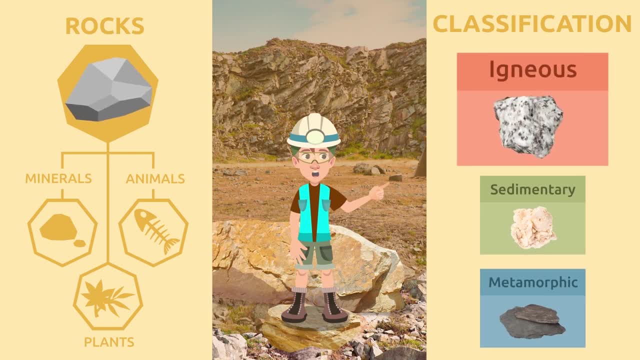 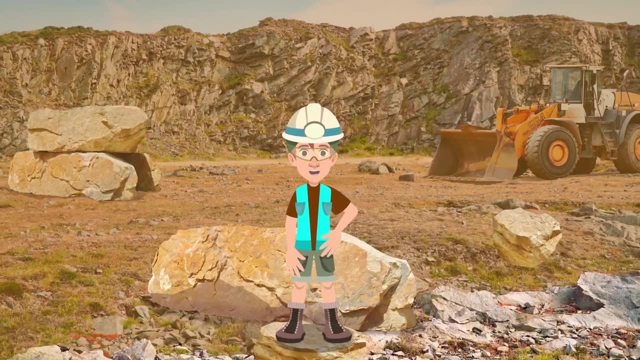 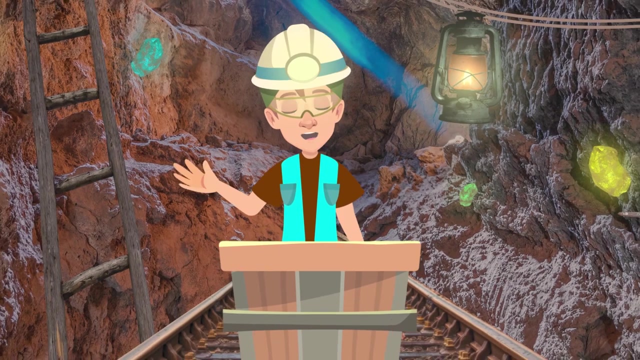 And that, based on their origin, we classify them as igneous, sedimentary and metamorphic Rocks are everywhere and play a major role in the world around us. Hello, friends, Ready for a new adventure? Today we're going to learn everything about minerals. 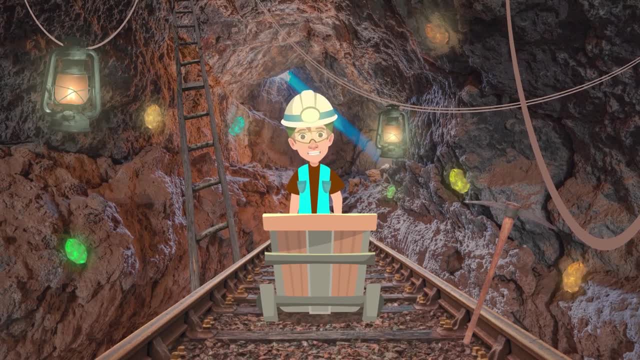 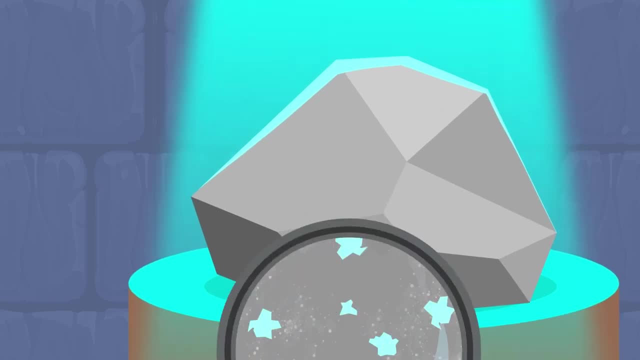 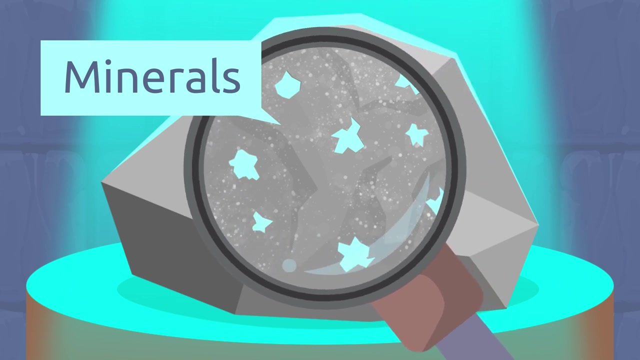 Do you know what they look like and how we use them? Let's find out together. We're going to use this magnifying glass to observe this rock. Can you see how it's formed by different elements? That's right, friends. those elements are called minerals and all rocks are made up of them. 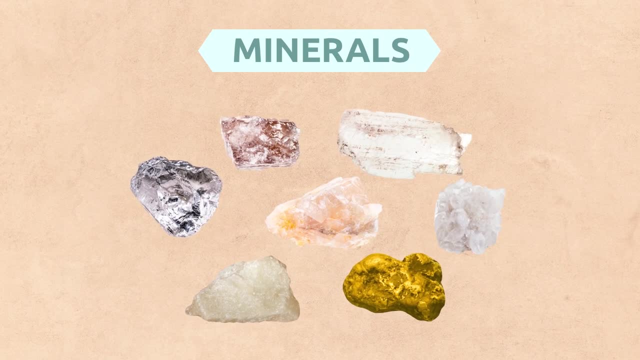 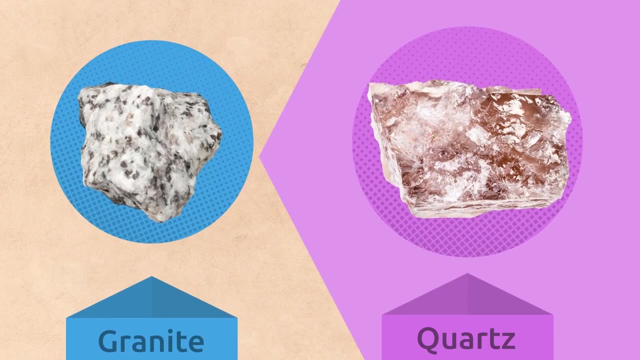 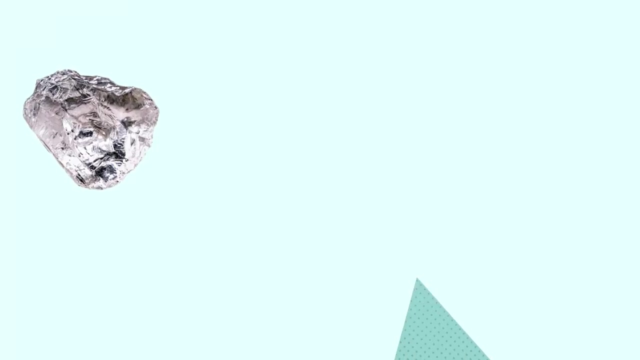 There are many types of minerals. Granite, for example, is a rock made up of a mineral called quartz. Marble is another rock made up of a mineral called calcite. Some well known minerals are diamonds, topazes, gypsum, talc and gold. 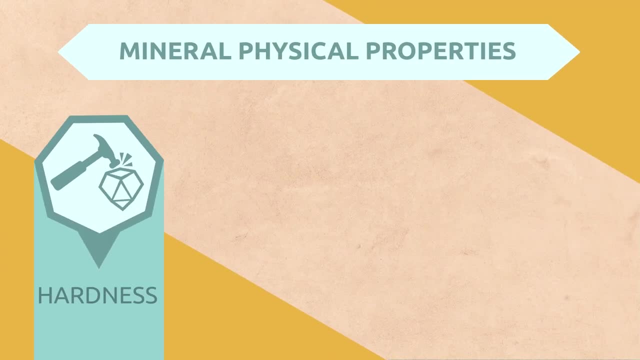 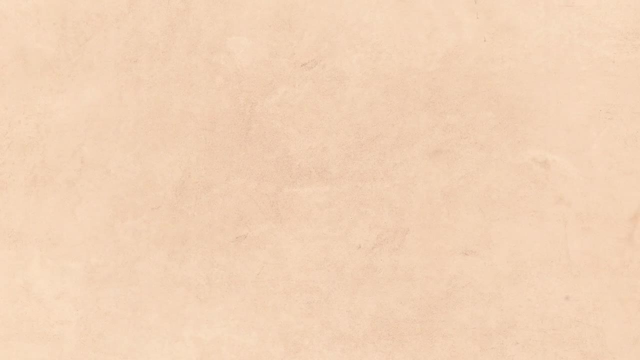 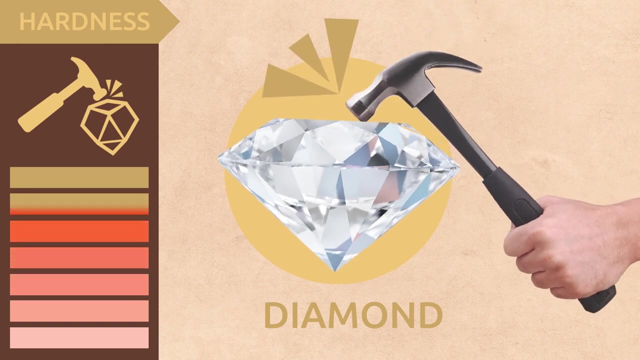 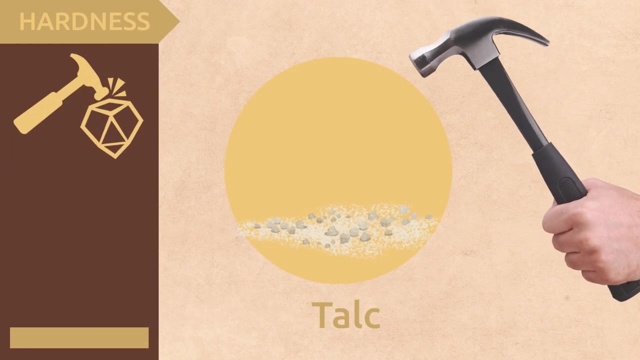 Minerals have the following physical properties: Hardness, shape, luster and color. Hard minerals are very difficult to scratch or break. Diamonds are very hard minerals, But talc flake's very stringy too is a soft mineral. The Mohs scale describes 10 minerals based on their 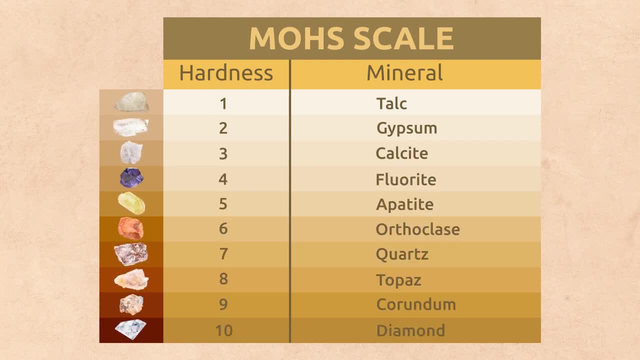 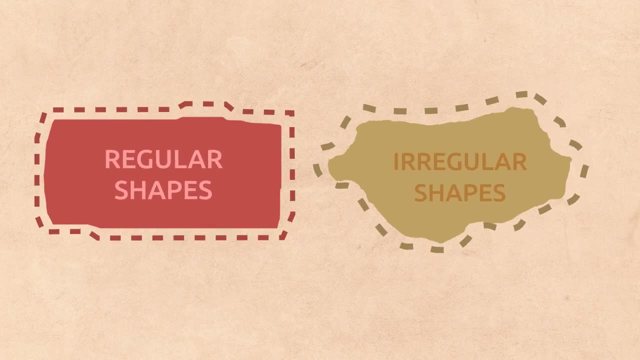 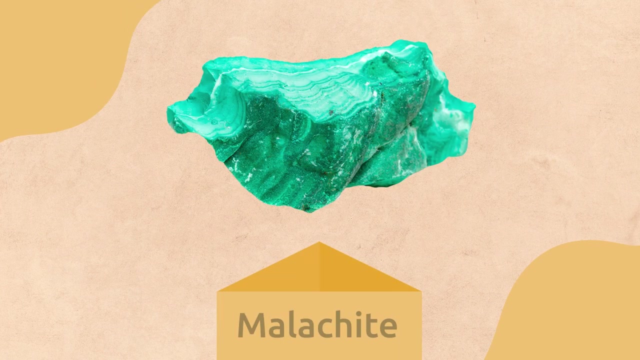 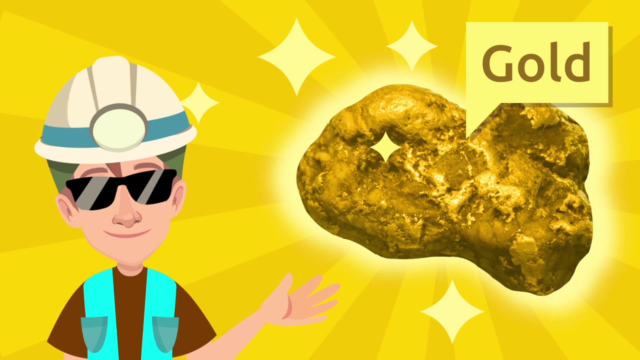 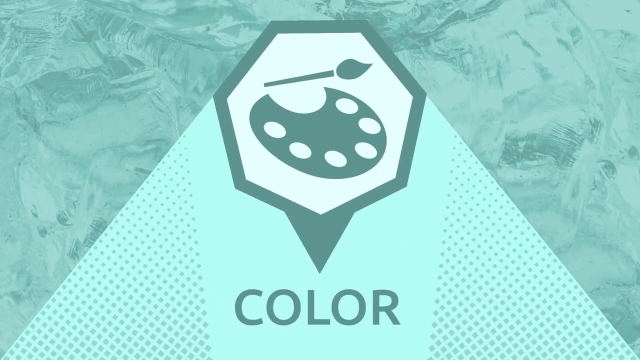 hardness, arranging them from softest to hardest. Minerals grow into different shapes, regular or irregular. Argonite has a regular shape, while malachite has an irregular shape. They look beautiful, Luster. There are shiny minerals like gold and others like talc, for example, with much less luster Color. 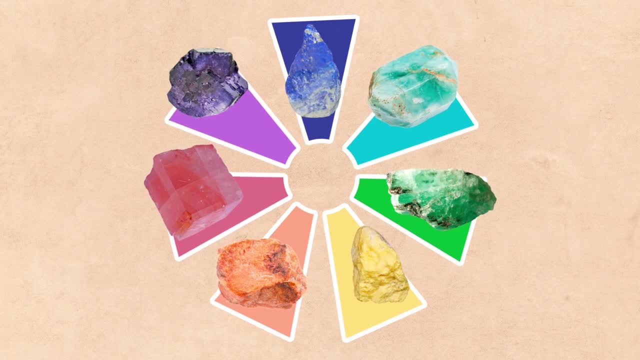 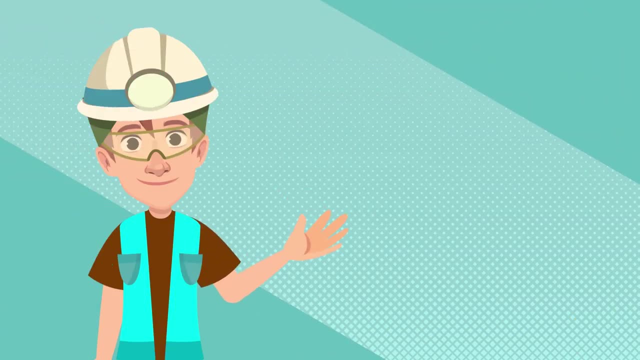 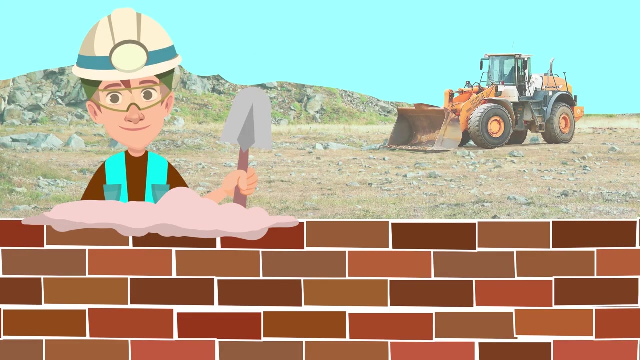 Each mineral has a distinct color. Emeralds, for example, are green, while sulfur is yellow. Did you know that we use minerals for many things? Let's look at some examples. Gypsum is a mineral used in construction. It helps to smooth out the surface of walls before painting.